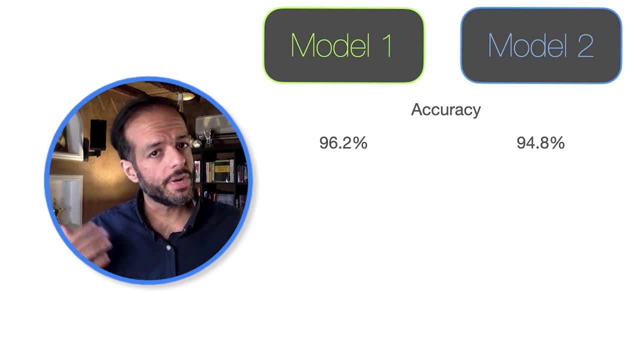 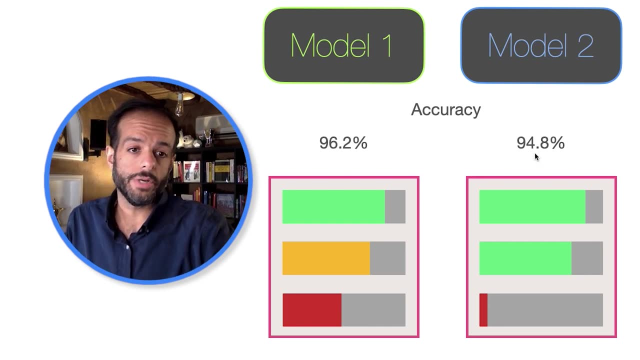 But then what if we look at them in a different way? What if we break down their, their capabilities, so to speak? One of them seems to so, the one on the right, with a lower accuracy, maybe, does better in two capabilities. let's say: 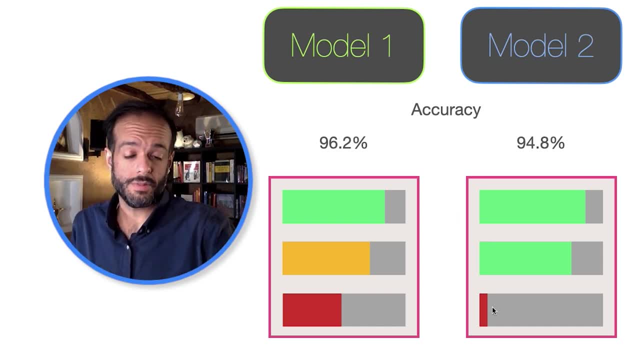 And maybe in our use case we care more about these two than this third one And in this scenario, the one on the right. despite having a lower accuracy or F1 or any sort of one number metric that does not give us enough of a picture about how the model really behaves. 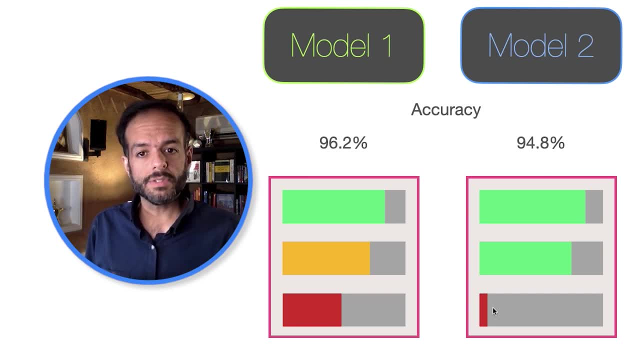 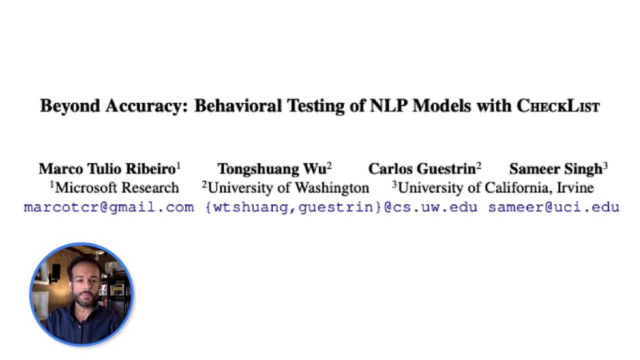 Using- Using our topic today, behavioral testing, we'll be able to get these scorecards that score models on multiple axes. So the paper we'll be discussing is Beyond Accuracy: Behavioral Testing of NLP Models, with Checklist by Ribeiro, Wu, Agustin and Singh. 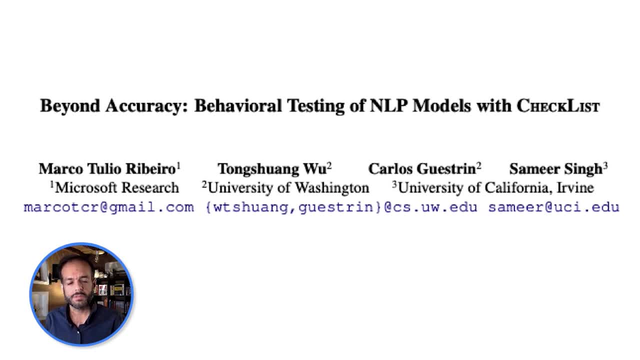 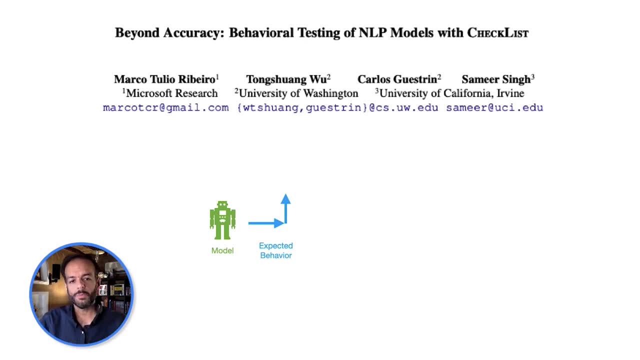 This is an- I think, an- ACL. it was the one- the best paper, I believe in ACL of last year And the basic idea is this: let's say we have a model. Let's say we have a small model. Let's say we have a small robot and we have an expected behavior. 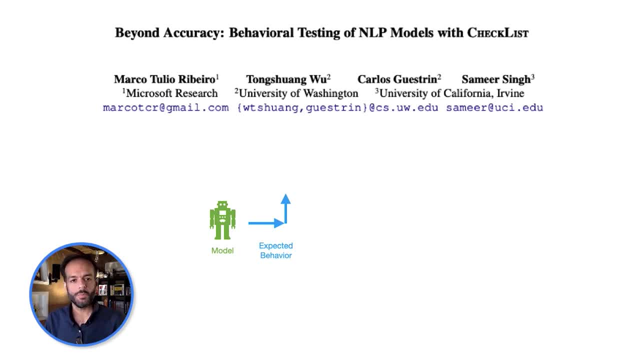 We expect that this, let's say, tiny robot will go straight and then take a left. How do we assure the quality, so to speak, of the behavior, that the model actually works, that the robot works how we expect it to do? 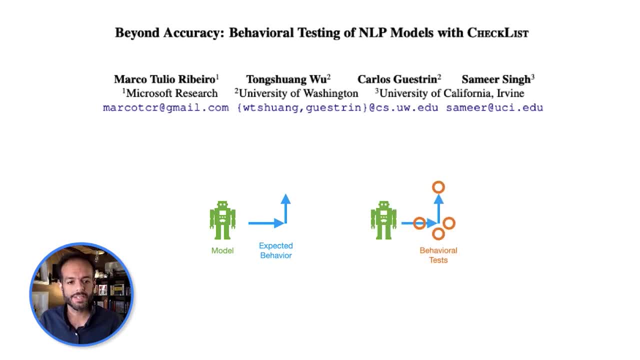 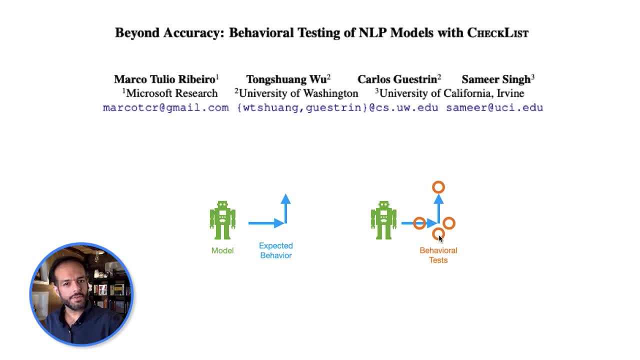 We can borrow this idea of unit testing from software engineering and say, okay, let's have a test here to make sure that the model reaches its end destination, where it's supposed to take a left turn. Let's have another test here to make sure. 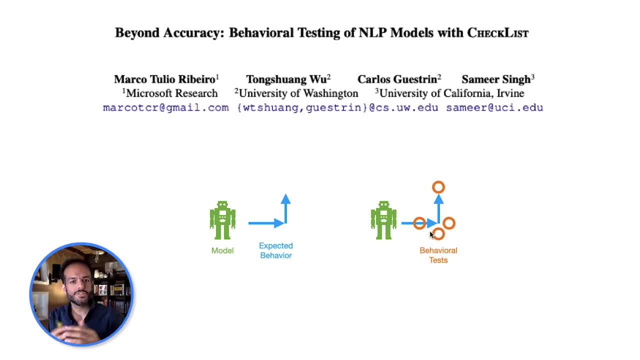 that it actually did turn left and not right. So you can just write these software tests to ensure that the behavior of your robot or your model is as you expect it, And you can run these tests numerous times, whenever you update it, whenever you get a new model. 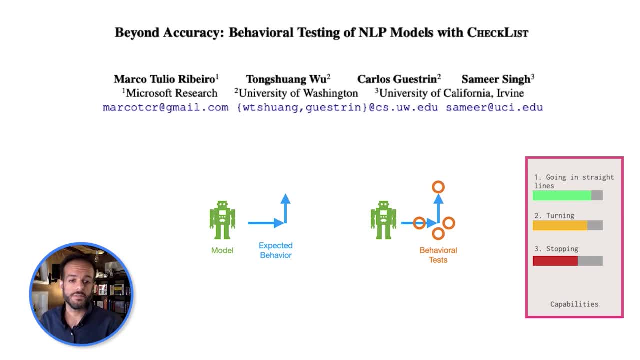 And then you can group these tests into capabilities, And so in this case we can say, okay, how well does this robot, let's say, go in straight line? So we maybe ran 10 different tests for it going in straight lines. 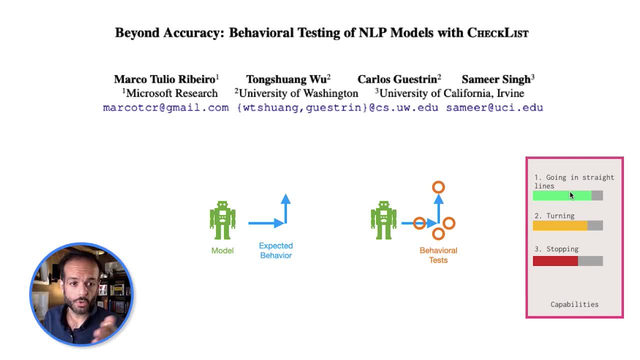 Maybe it succeeded in nine of the 10. And so we have a score for this capability. How well does it do in turning and stopping, So on and so forth? So this is a miniature model example, but then let's look at how that can be done in NLP. 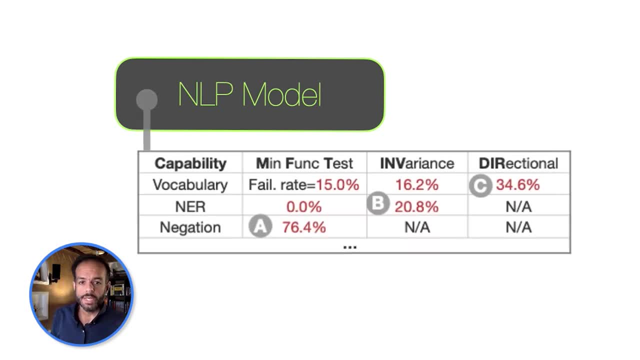 And that's the topic of the paper: NLP models. So this is an example of a scorecard directly taken from the paper. Let's look at the first column on the left. So instead of turning and stopping, we have actual linguistic capabilities. 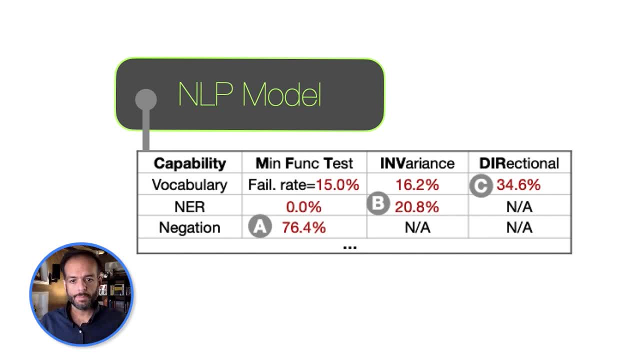 that models are expected to have, So how large their vocabulary is. Negation is the one that we're going to go into a little bit more, And then we'll focus on this, the second column. first, the minimum functionality test. Don't worry about the other two for now. 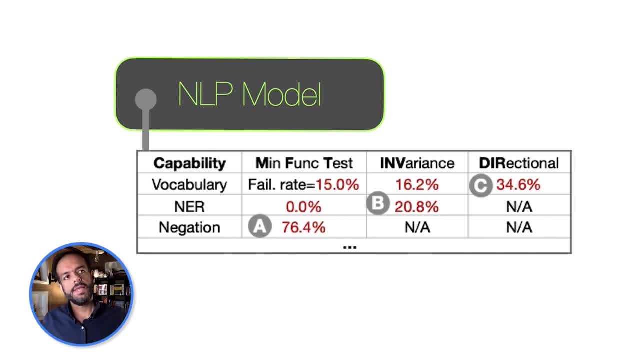 We'll get to them. So negation is important And the main example of NLP models we'll talk about here, and the one they discuss in the paper, is sentiment analysis. So, given a sentence, is the sentence saying something negative or something positive? 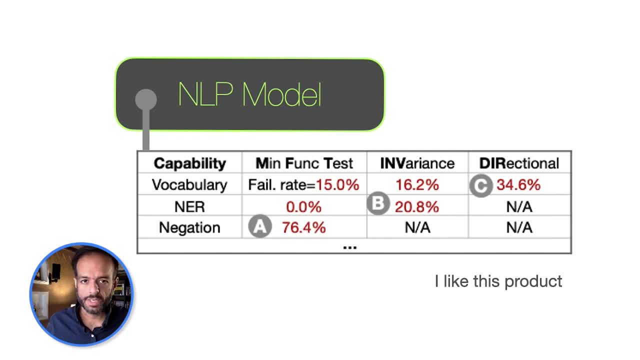 Now, if you have a sentence like this, saying I like this product, this is a positive sentiment. This is clear. But then what if you add: I don't like this product. It's exactly identical except for one word that does negation. 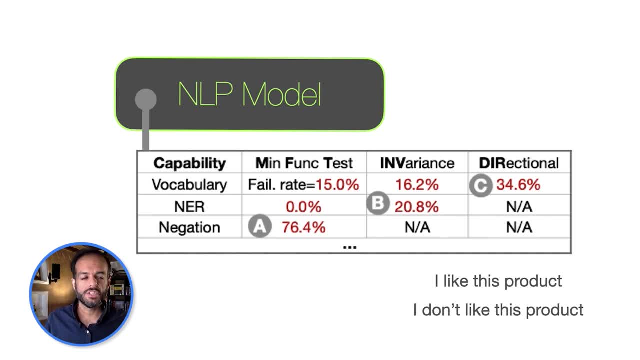 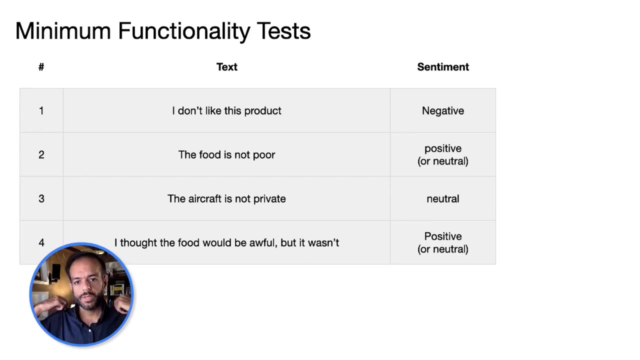 And if a sentiment analysis model does negation well or does not do it well, that affects its final sort of goal and its performance. So let's see how we can test a negation using something like like checklist, Basically the the unit tests in the machine learning domain. 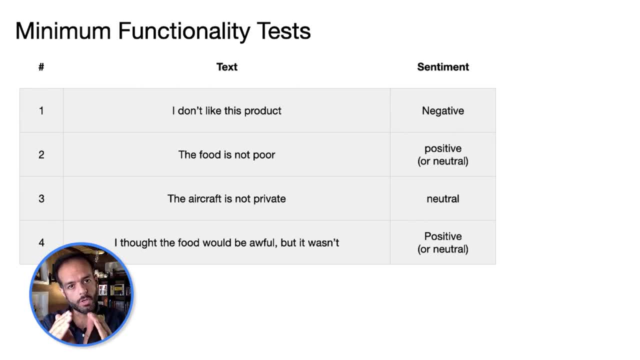 would be a small dataset that we carved out that we know handles this behavior. So we have examples of inputs and we have a label associated with them. So here, for example, we want, I don't like this product, So this would be a negative sentiment example. 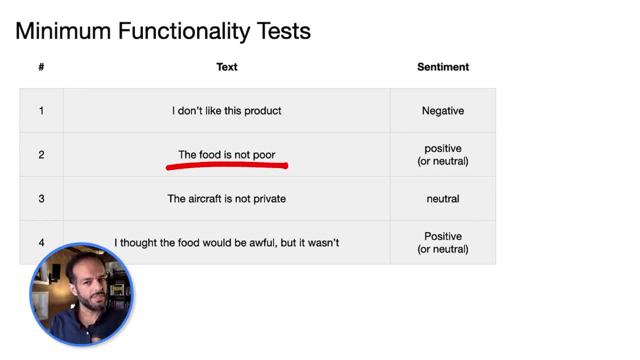 The food is not poor, So it's not bad. So it's either positive or neutral, based on you know, does this model have a neutral classification, or is it just positive, negative? And then you have something that's: the aircraft is not private. 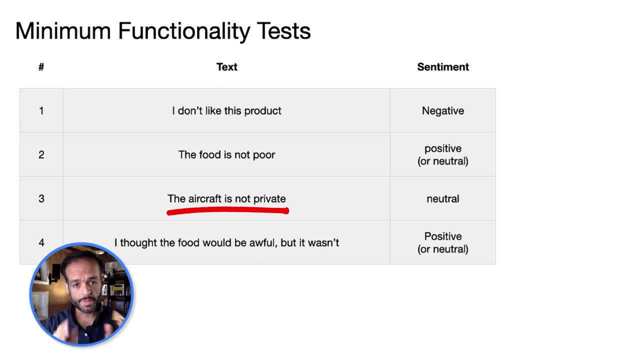 So the sentence itself was neutral, but then you negate it, the neutrality. It should still be neutrality, And so that should still be neutral. So how do we run the test? We feed the model, the texts, and we have it make predictions. 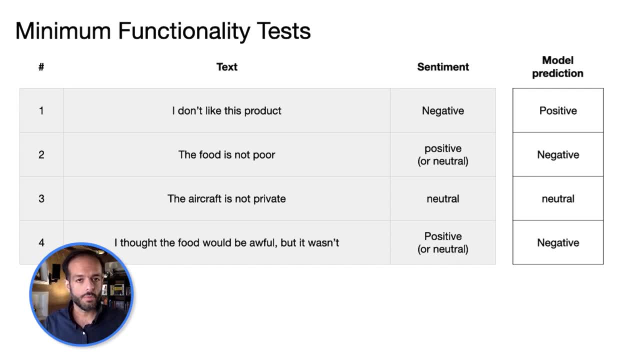 And then if we have a model making B these predictions, we just compare them with the labels. This one got three wrong and one correct, And so that's a 75% failure rate, And this is a functionality test that tells us how well a model 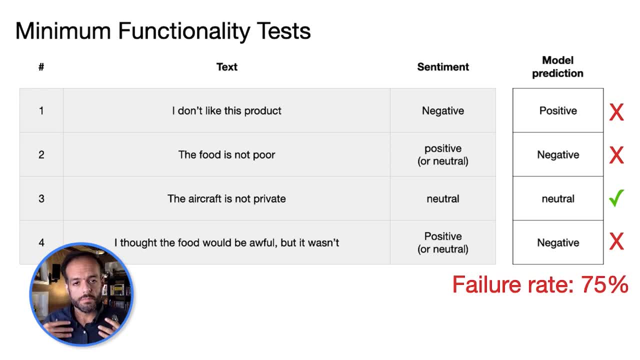 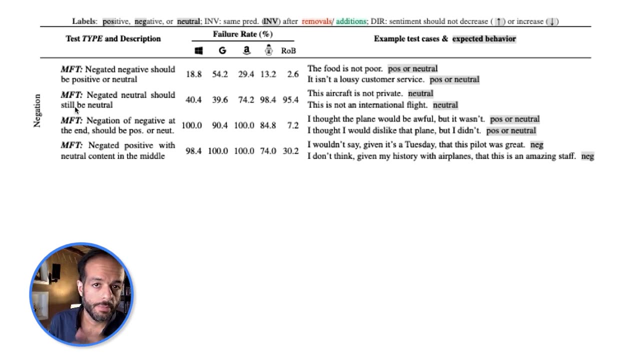 does on negation. And then you're not limited to only having four. you should probably have 50 or 100 or a lot more examples to test things. This is an example from the paper. So here you can see MFTs are minimum functionality tests. These are the tests that look like small data. 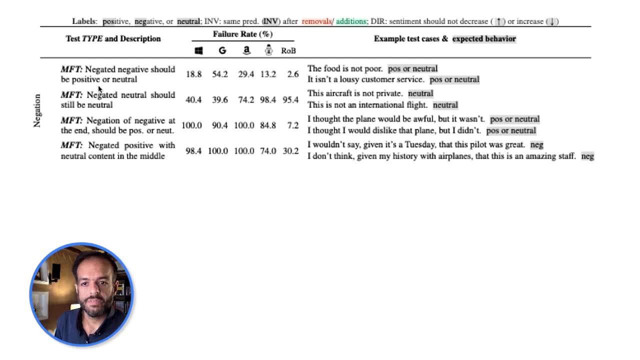 sets. So this is, let's say, test number one: Negated, negative should be positive or neutral, And here they have examples. So the food is not poor should be positive or neutral. And then here they evaluate five different models. So I think this is a BERT, this is Roberta. 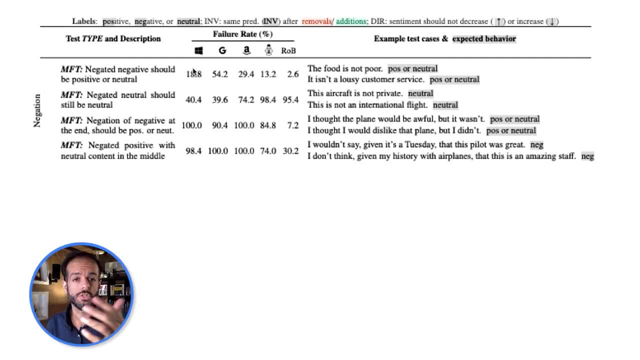 both trained on sentiment analysis. And then these are commercial models. So this is a sentiment analysis model from Microsoft, From Google, from AWS, And these are their failure rates. So under this test there are, let's say, you know, 20 or 30 or 50 examples And this is the failure rate. So the lower these 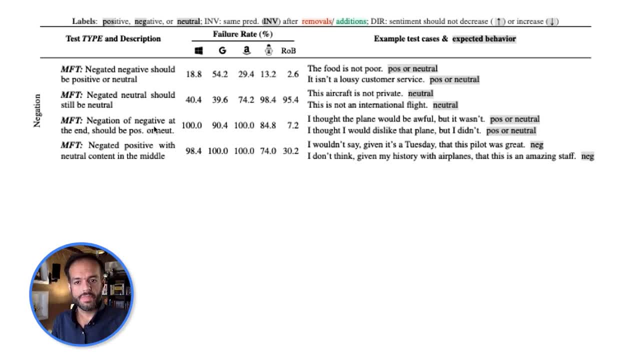 numbers are, the better this model would be. And then you can see tricky examples here, like negation of a negative at the end should be positive. So I thought the plane would be awful, but it wasn't. So all of the models except for Roberta. 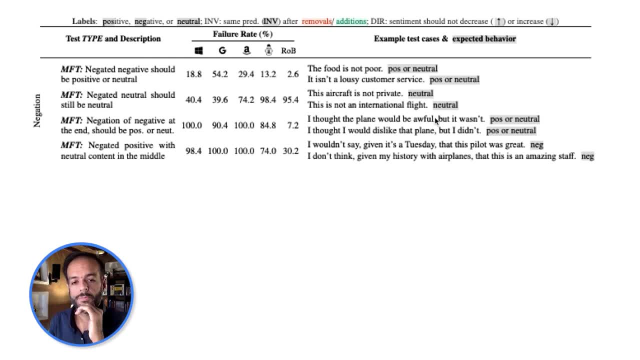 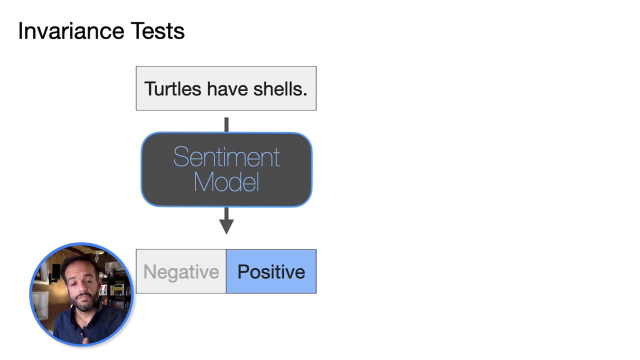 find these are very difficult, So they fail the majority of times. So this is an interesting way of how you can evaluate, let's say, models and quality assure them as part of, let's say, CICD setup. The second type of test is an invariance test, And the example here is to say: 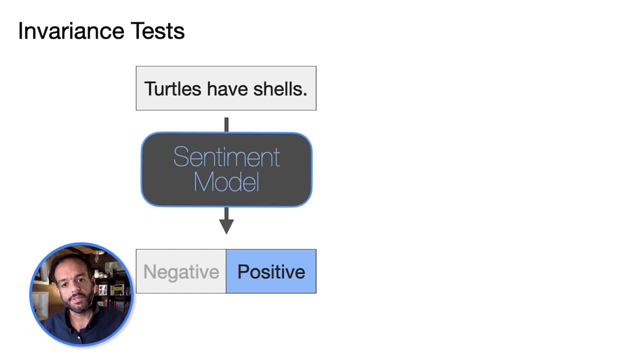 let's say we have a neutral or a positive sentence, like, let's say, turtles have shells, If we change the example in a way that does not change sentiment, So if we say feet instead of shells, the prediction of the model should: 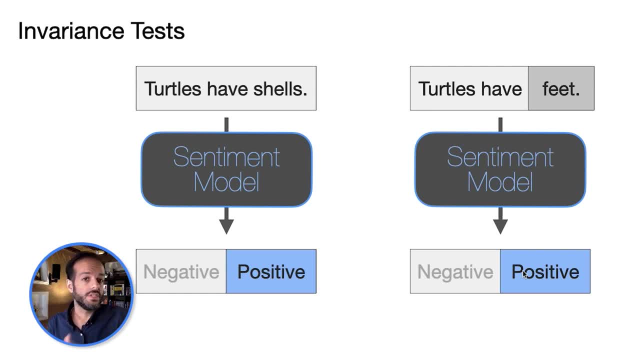 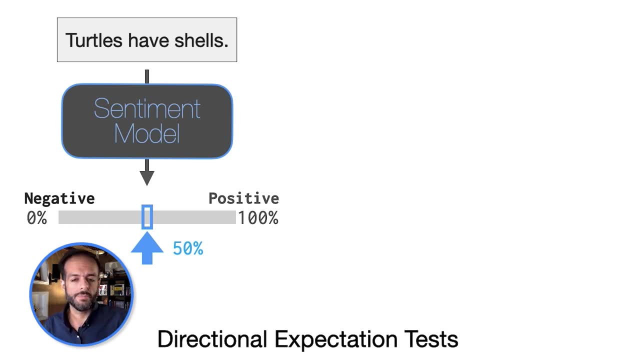 not change. The class should not flip. So this is an example of type of tests. And the third type of example is called a directional expectation test And it goes like this. So we have a sentence and then we predict it with the model, And the model says: 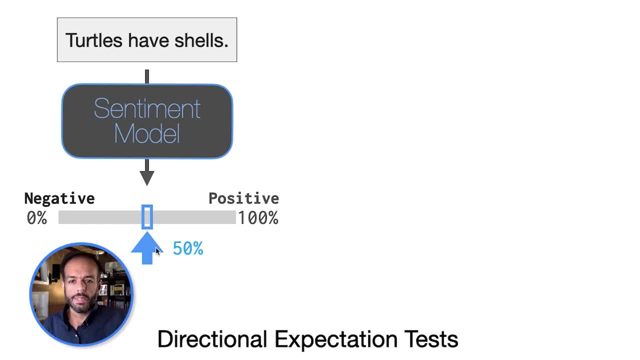 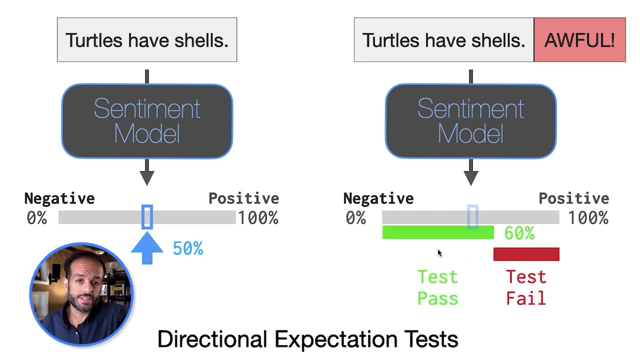 okay, this is 50% positive, So it's between positive and negative. Let's say we add a negative portion to the end of the sentence. How would the model react? Would this score increase or decrease? So if it decreased, the test would pass. If the model says that this sentence 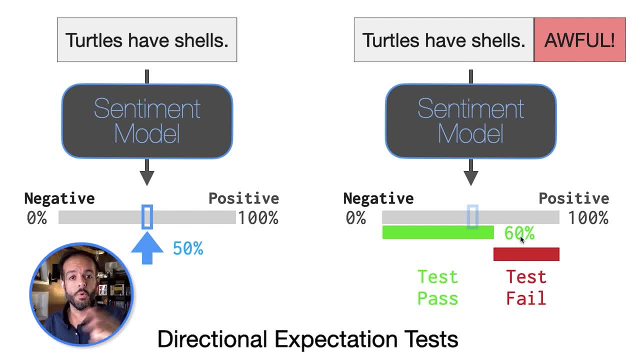 including the word awful- is actually more positive than this one, then that's a test failure. So the idea here is that these are kinds of tests that if we perturb or change the input in a way, know should take the prediction in one direction, that the model does not go the other way. 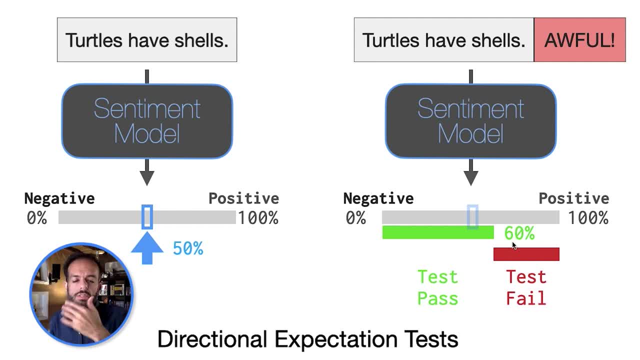 It can go up, maybe 10%. so this is up to you, but this is the default that they work with, just to account for just the general behavior of models and how they do that. So it can go up a little bit, but not too much. 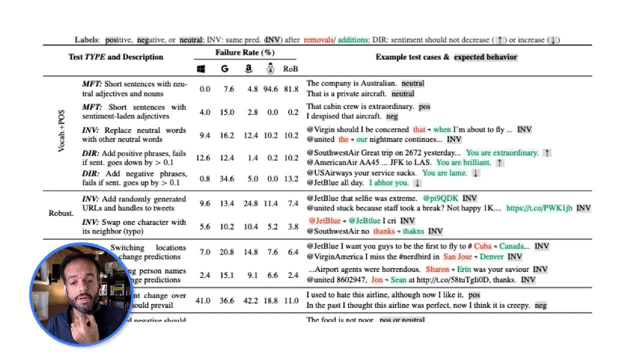 Here is a scorecard in more detail, sort of comparing the various capabilities. So here you have the prior speech and vocabulary and then you have the minimum functionality test, what it looks like, And so this is short sentences with neutral adjectives and nouns. 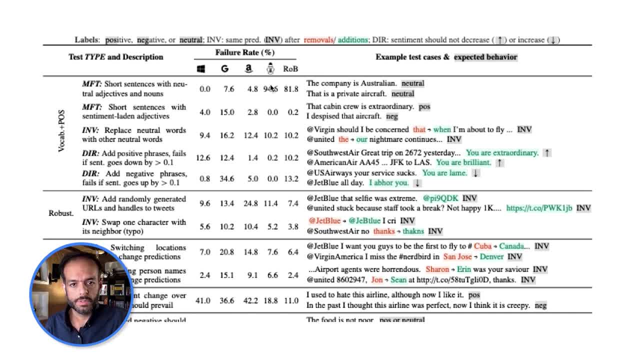 A lot of them get them correctly, except this part fails at these for some reason. And then here you have invariance tests, So replacing neutral words with other neutral words. So if you have this, let's say: maybe this is a tweet. 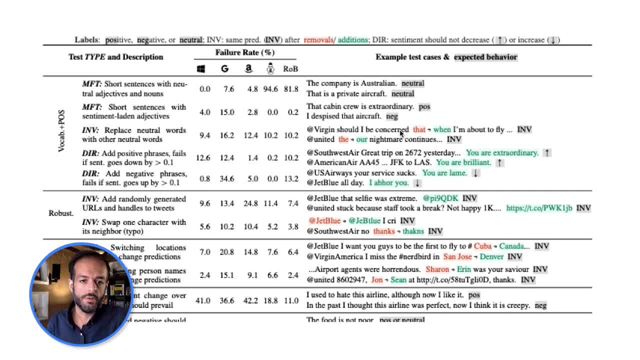 So should I be concerned when I'm about to fly? Originally it was. should I be concerned that I'm about to fly And then that has a certain prediction? Then if we switch that to when the prediction shouldn't change, And so there's a low failure rate across the models, but then there's still something. 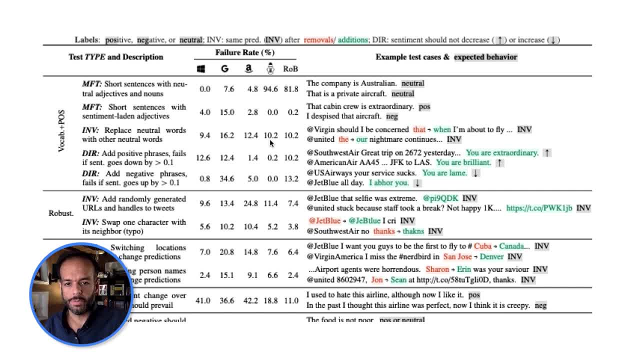 they can probably update them to have even lower failure rates. And then you have the directional expectation test here. So if you add a positive phrase, make sure that sentiment that the score should be higher, does not go down, that it's not indicated to be more negative, so to speak. 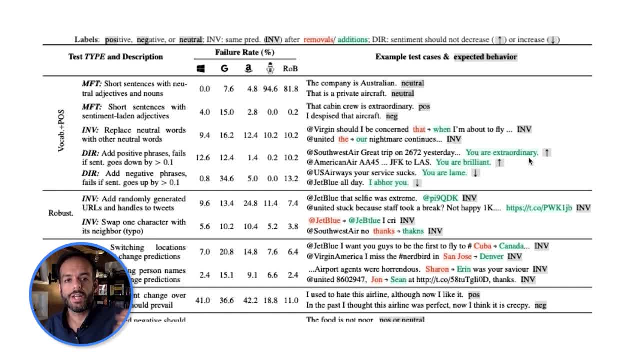 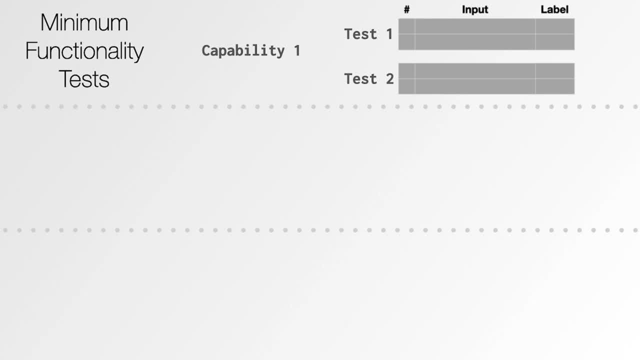 So they add: you are extraordinary, And so the score should actually go up and not go down, And so this is this kind of test. So, to recap, the first kind of test is the minimum functionality test. This looks like unit tests. 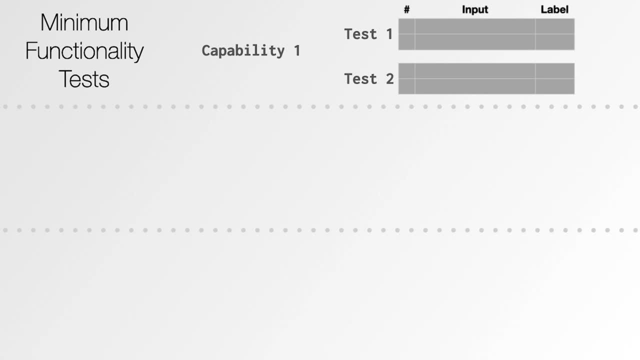 They're small data sets that test specific capabilities. Then we have the invariance tests, where we perturb, change the inputs in a way that we know shouldn't It does not affect the output, and we measure if it does or does not. 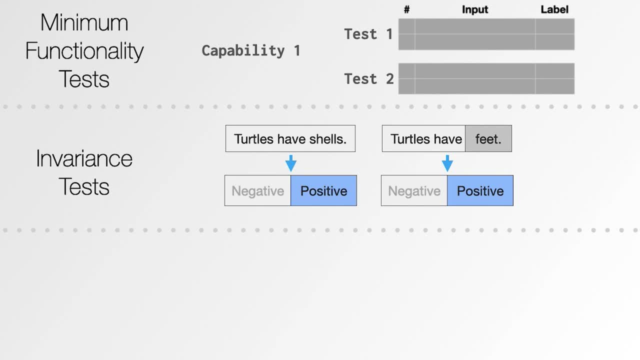 And the checklist open-source library that they provide with this paper includes templates that allow you to generate these kinds of perturbations for the input. Then we have the directional expectation test, where the idea is, if we make a perturbation to the input that is expected to shift the output one way or another, it's for us to. 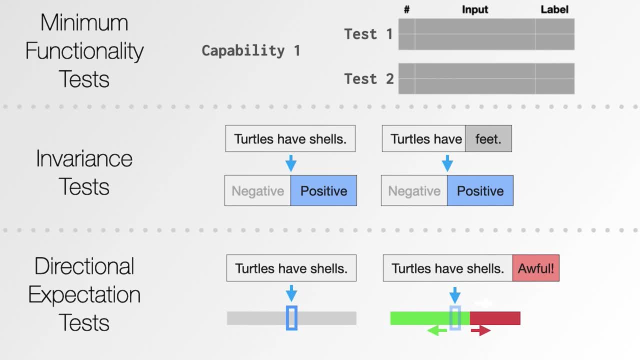 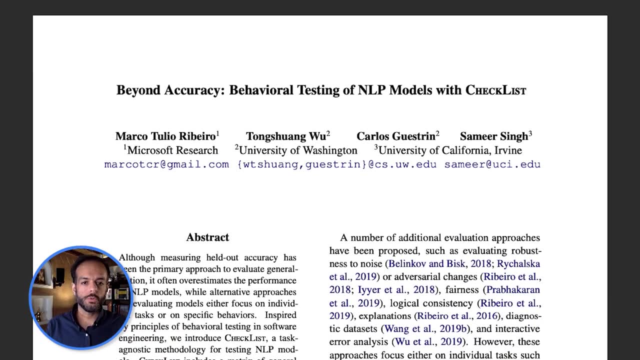 make sure that it goes the way that we're expecting And not the other way, other way. So adding a negative word shouldn't make the prediction more positive. So this has been your intro to behavioral testing of NLP models with Checklist. I invite you to read the 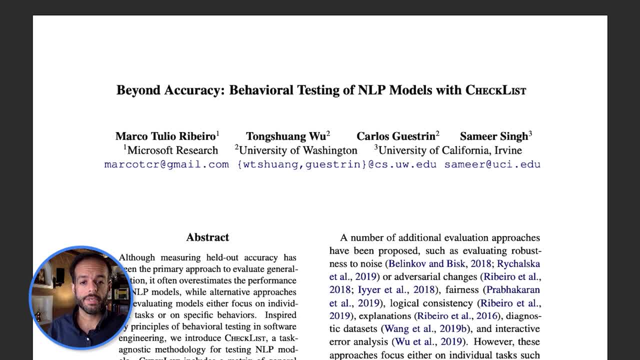 paper. check out the GitHub library- There are links down in the description- And then I can see several scenarios where. So we talked about where this can be used. So we talked about comparing models, But I also am excited about having this just as running on, If you have a. 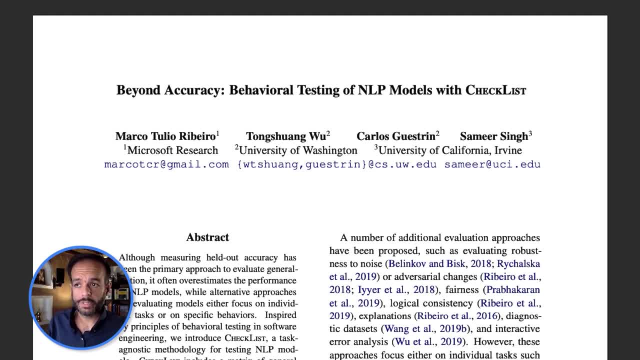 model in production. it's good to make sure that the next update or the next time you retrain it, that one of the core capabilities that the model should be able to do has not degraded, Or that, if it did degrade, that you know about it. It's just to carry over these practices. 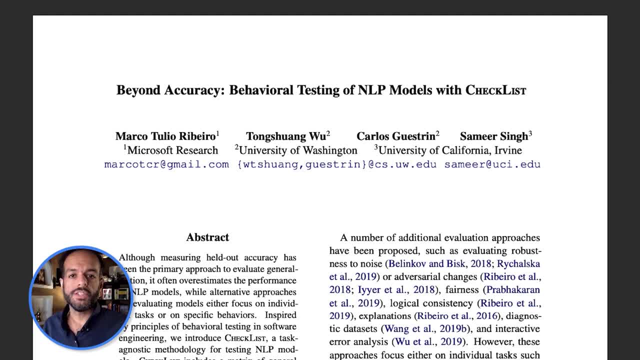 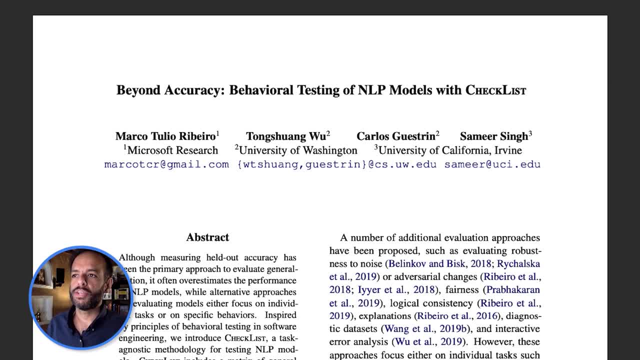 Robust Because I've seen it. I've seen companies that struggle because of not investing enough in automated testing and in software tests and unit tests, So a lot of the engineers spend a lot of their times bug fixing And I've seen frustrated CEOs. 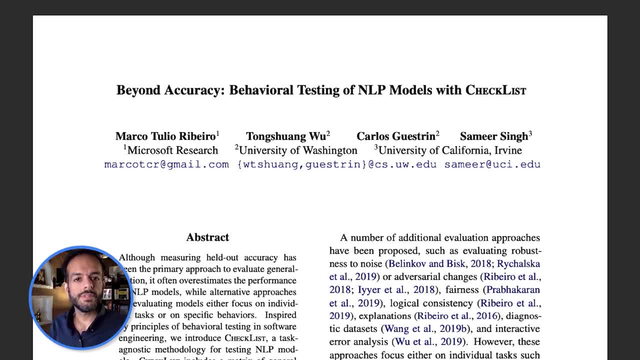 by the speed of the development that a lot of these software practices are able to help an organization that is growing, And the more we adopt that in machine learning and in machine learning practices, I think that that'll lead to better organizations and better practices and operations. Thank you for watching and see you in the next video. 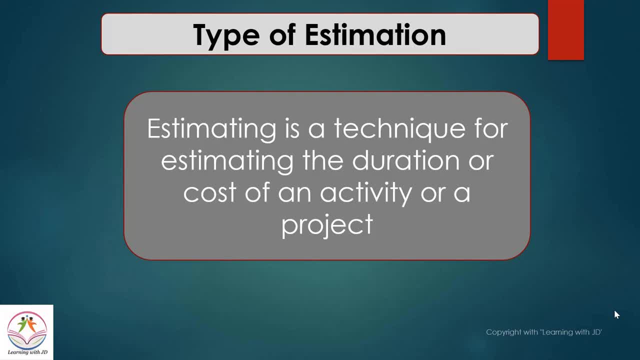 Hi guys, welcome back to learning with JD. So in today's session we are going to talk about the type of estimation. What do you mean by estimation? Estimating is a technique for estimating the duration or the cost of an activity or a project. 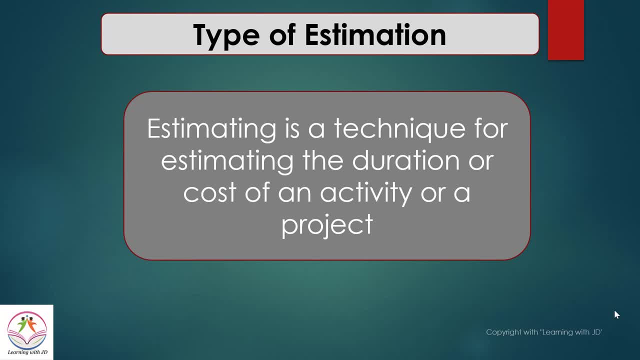 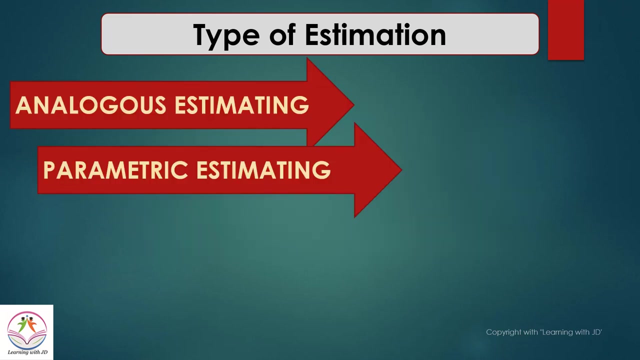 So understand that when you are in your planning stage, there are various tools and techniques that you used for estimating what will be the approximate duration in which you will complete an activity or a project and how much is the cost that you need. So there are four kinds of estimation techniques. We are going to see all of them today: Analogous estimation, parametric, three point estimation and bottom up estimation.